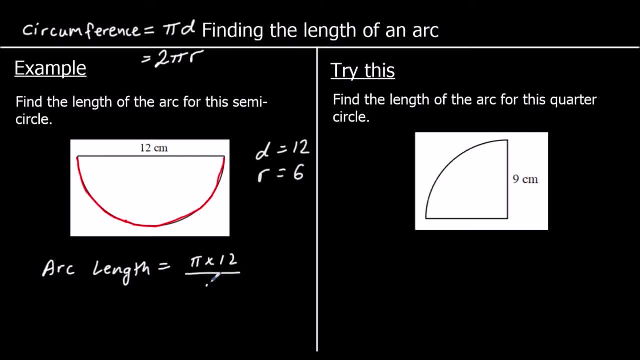 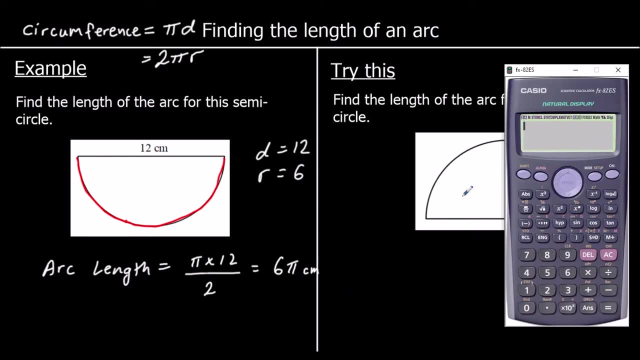 divided by two, because we've got half of a circle. So that's 12 pi over two, which is six pi, And it's in centimeters. If we wanted to give our answer as a decimal, we could type six pi into the calculator and press the S to D button and we'll get 18.8495 and so on. 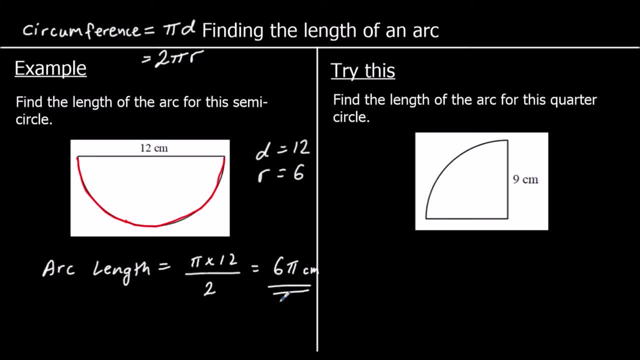 But six pi centimeters is a perfectly good answer, Okay, one for you to try. So you've got a quarter circle. Can you work out the length of the arc? So, again, the arc is part of a circumference. So we have a quarter of a circle, So we can work out the circumference of the whole circle. 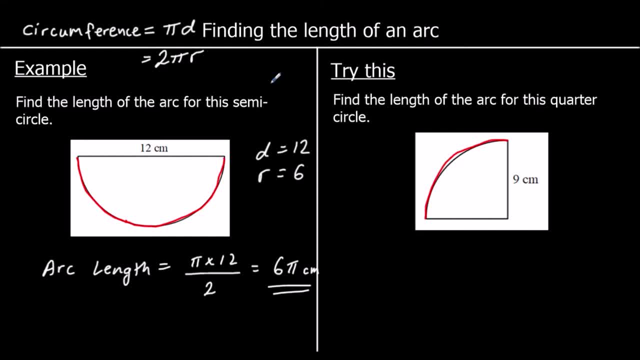 and divide it by four, So the circumference of the whole circle. this circle's got a radius of nine or a diameter of 18.. It doesn't matter which one you use, you will get the same answer. So if I say the arc length, 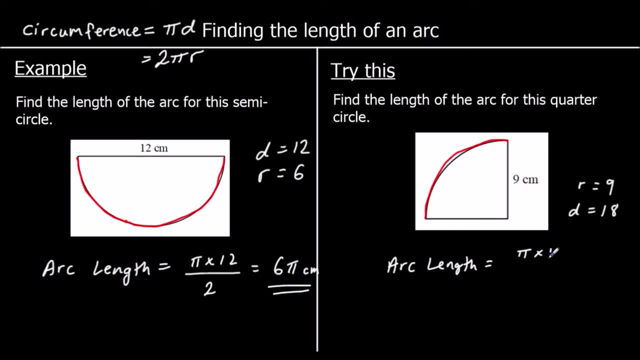 is pi times the diameter divided by four, So 18 pi over four, which I can simplify to nine pi over two. And again it's in centimeters. It's a length. We measure it in centimeters And if we wanted to give our answer as a decimal, we could type this into the calculator. 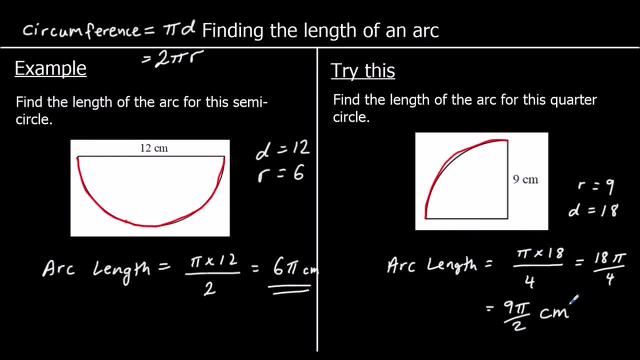 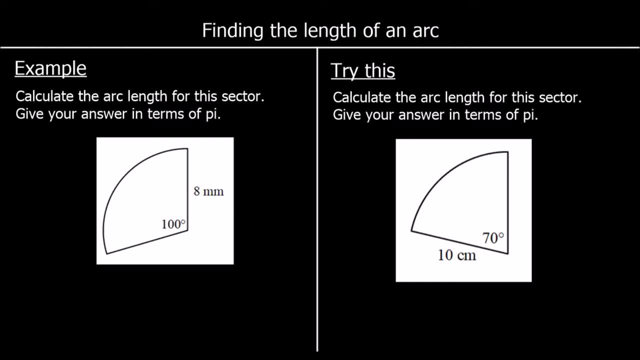 and we will get a decimal out. Here's another example. This time we've got 100 degrees. So we've got 100 degrees out of the whole circle, which is 360 degrees. So I'm going to say I've got 100 360ths. 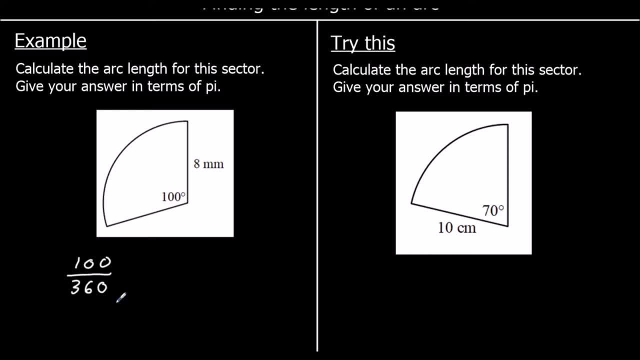 of the whole circle. That's the fraction I've got. So to find the arc length I'm going to do 100 over 360 times the whole circumference. So I want this fraction of the whole circumference. so I do this fraction times the whole circumference And again I can use pi times d. 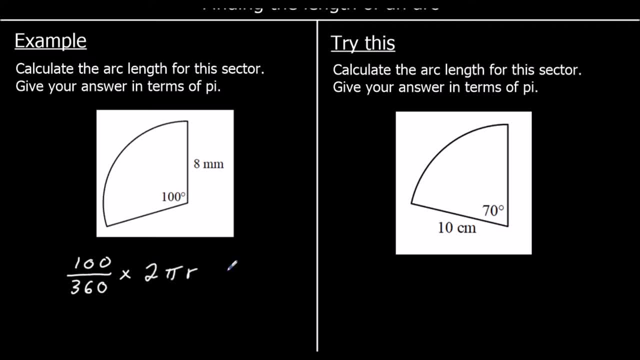 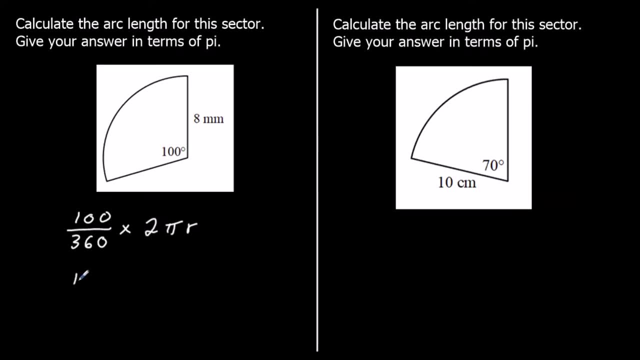 or 2 times pi times the radius. It doesn't matter which formula you use, they are the same. So the radius is 8 this time. so 100 over 360 times 2 times pi times 8.. And we can type this into the calculator. 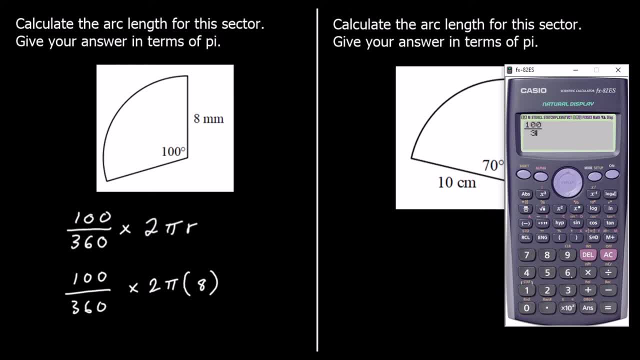 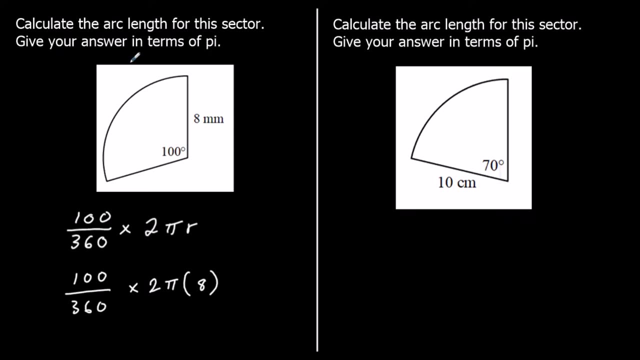 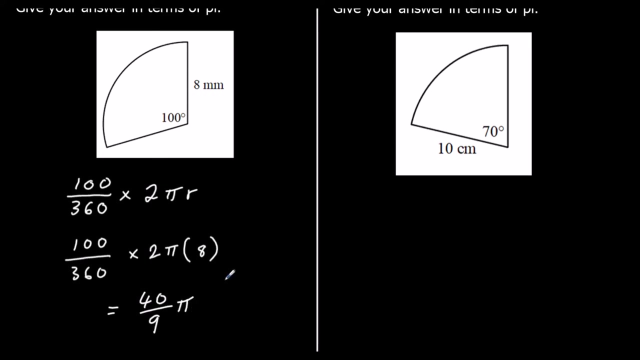 So 100 360ths Times 2 times pi, times 8. And I've got 40 over 9 pi. So I'm going to leave my answer in terms of pi. So it's 40 over 9 pi and it's a length and we're measuring it in millimetres this time. 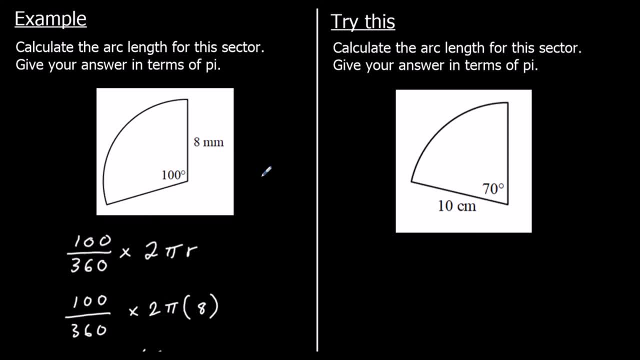 Okay, one for you to try. So give this one a go. So again we're calculating the arc length. So what fraction of the circle have we got? We've got 70 out of 360. And we're going to times that by the circumference of the whole circle. 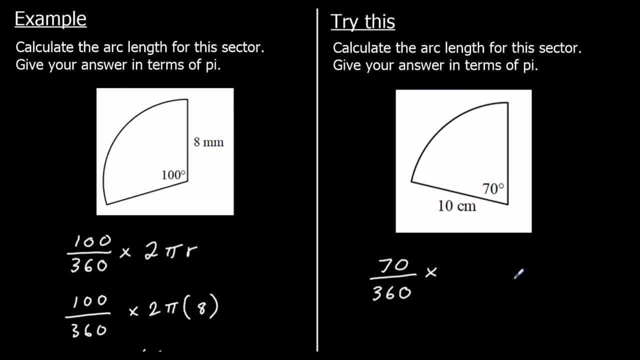 So we want this fraction of the entire circumference. So we have 2 times pi times r or pi times d, If the radius is 10, the diameter is 2 radiuses, which is 20.. So 70 over 360 times pi times 20.. 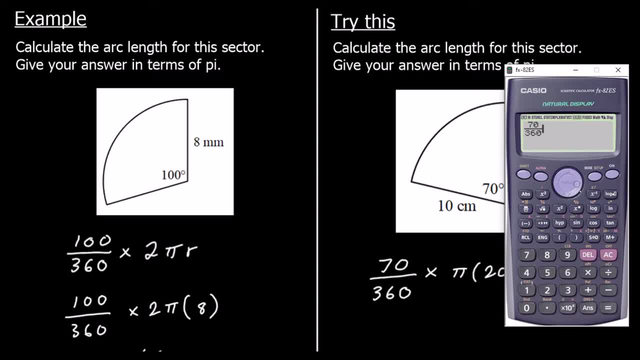 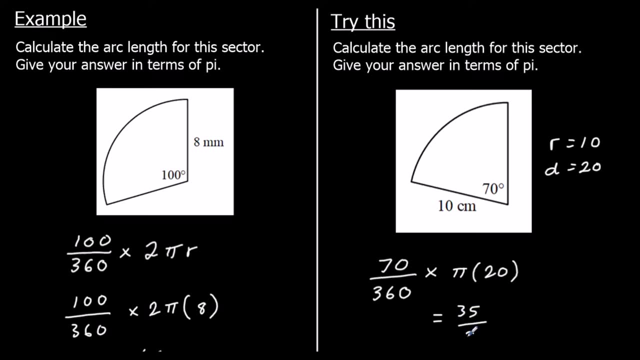 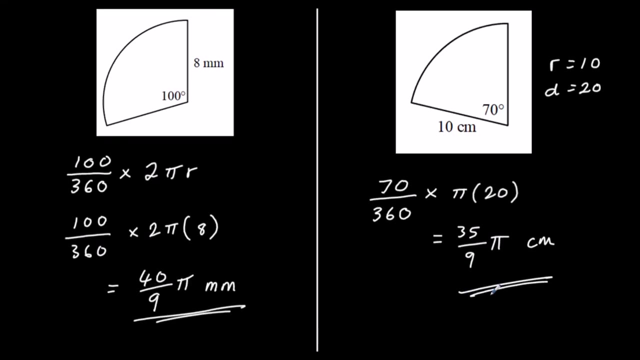 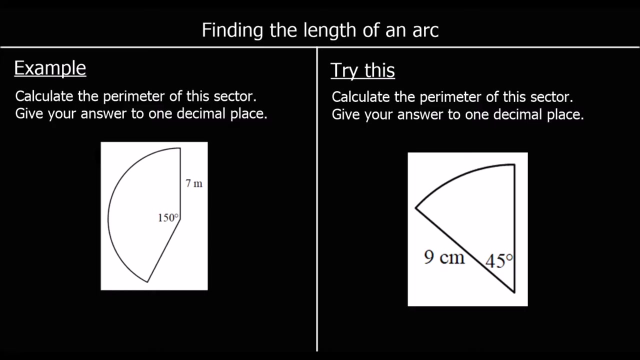 70 over 360 times pi times 20.. So 35 over 9 pi. Yeah, And that's in centimetres. Here we have another example. This time the question says: calculate the perimeter of the sector. So this shape is a sector. 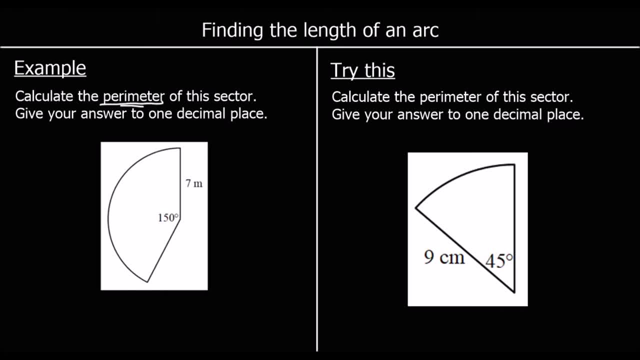 And we need to calculate the perimeter. And we need to calculate the perimeter of the sector. So this shape is a sector of it. so we're going to find the arc length and we're going to add on two radiuses. so we're going. 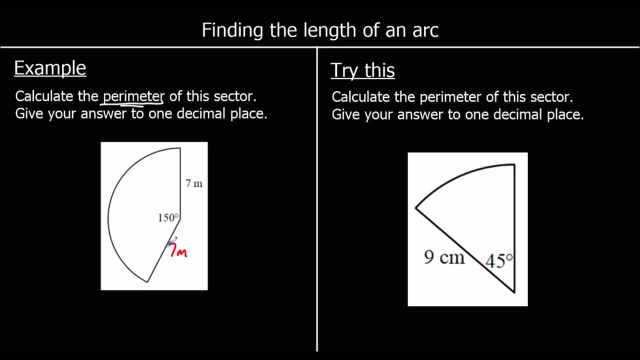 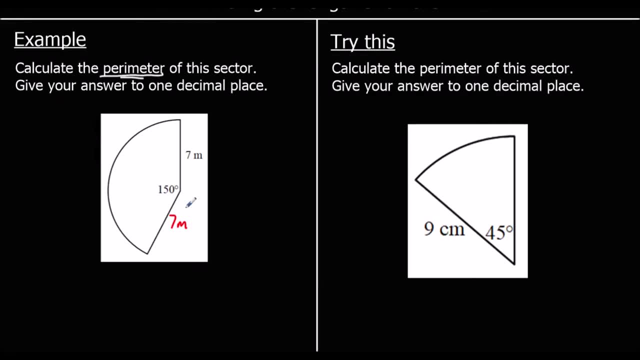 to have an arc length plus two radiuses. so let's find the length of the arc. so we've got 150 degrees out of 360. so we've got 150 360ths of the circle. that's the fraction we've got. so we want that. 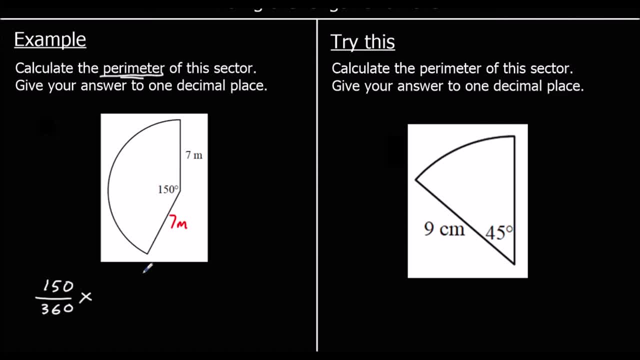 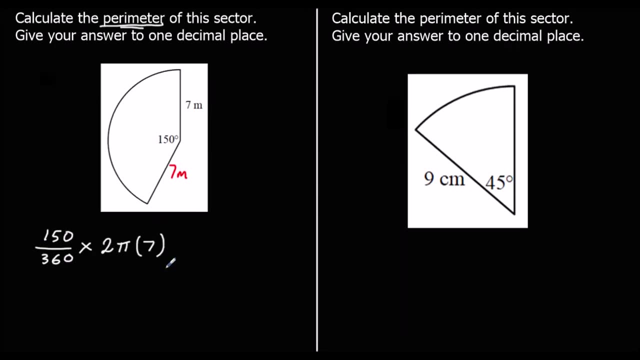 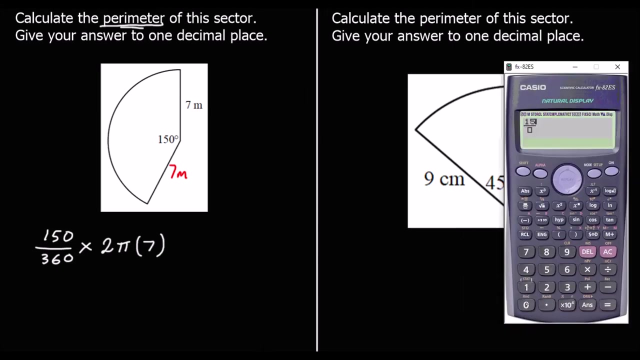 fraction of the circumference, which is either 2 pi r, 2 times pi times the radius, which is 7, or pi times diameter, which will be 14. so we can type this into the calculator to find the arc length. so it's 150, 360ths of 2 times pi times the radius, which is 7. 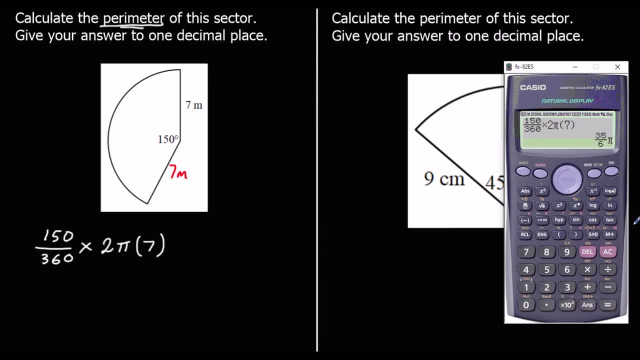 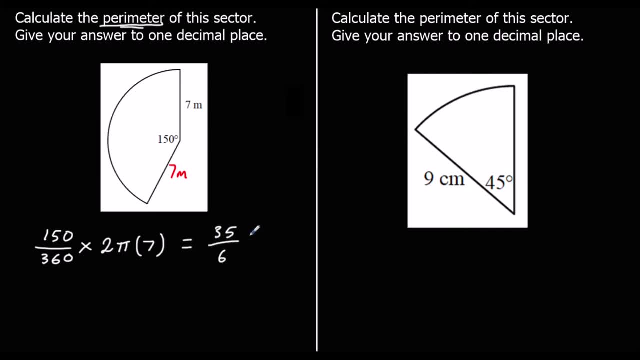 so that's 35 over 6 pi. so i'm going to leave that number in the calculator and i'm going to add on my two radiuses. so it's going to be 35 over 6 pi plus my two radiuses. so to my answer. 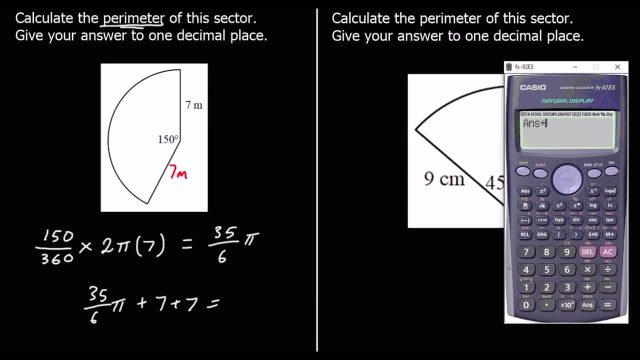 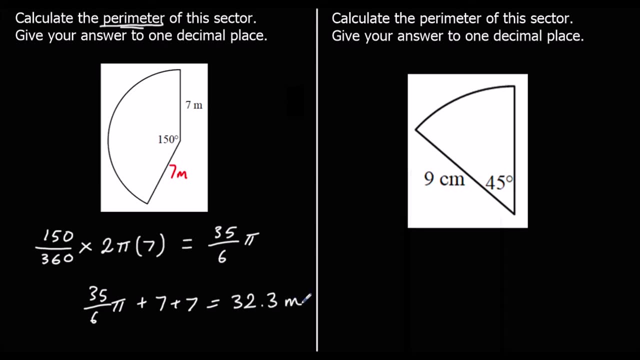 i'm going to add on two sevens and to one decimal place. given my answer to one decimal place, i've got 32.3 and it's in meters. 32.3 meters the perimeter length, so it's measured in meters this time. and one for you to try so calculate the perimeter. 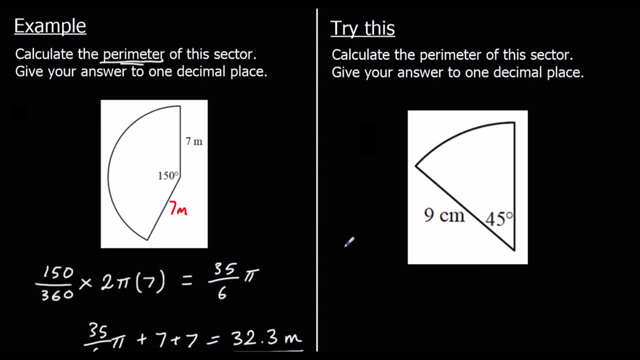 of this sector and give your answer to one decimal place. so again we're going to find the arc length, and then we're going to add on two radiuses to find the perimeter, so the arc length. and then we're going to add on two radiuses to find the perimeter, so the arc length. 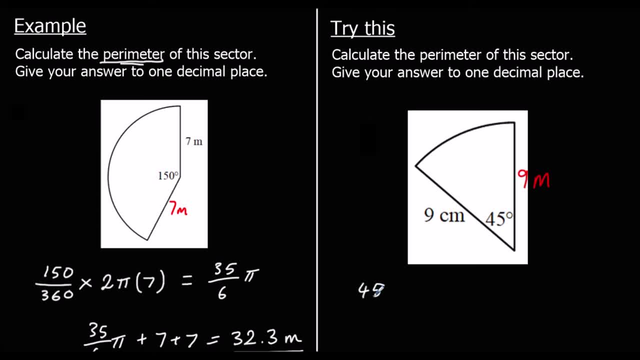 is going to be 45 360ths, that's 1, 8th. so we want 1, 8th of the circumference of the whole circle, which is either 2 times pi times the radius, so 2 times pi times 9, or pi times diameter, which would be pi times 18, so 45 360ths. 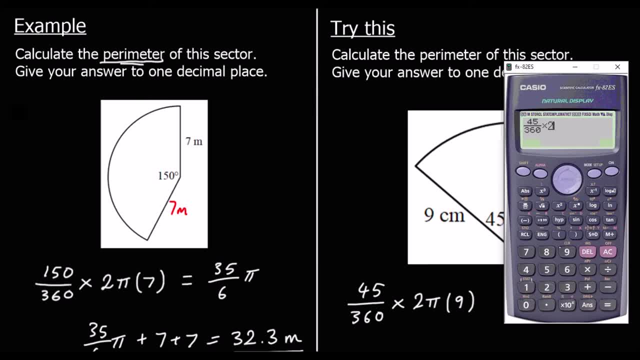 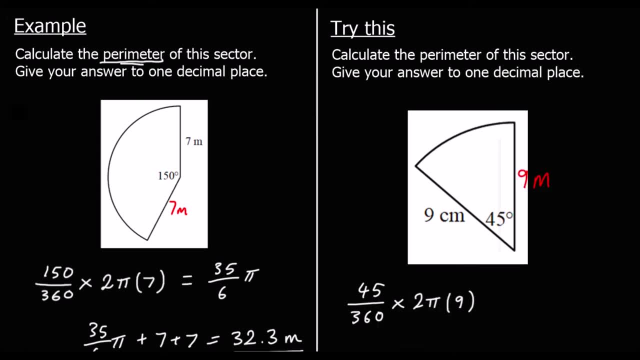 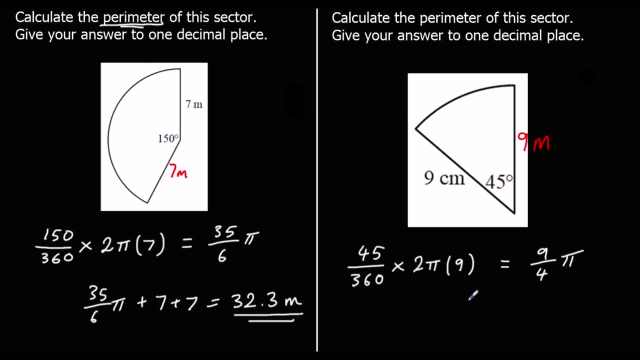 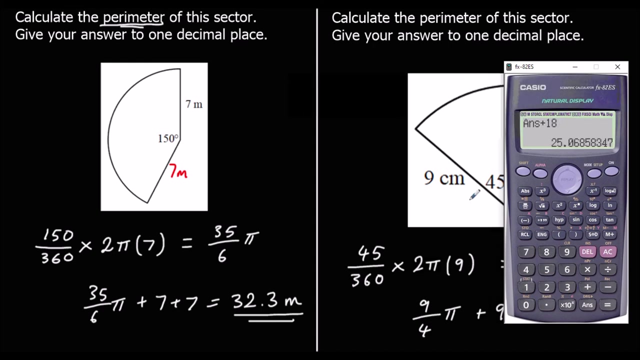 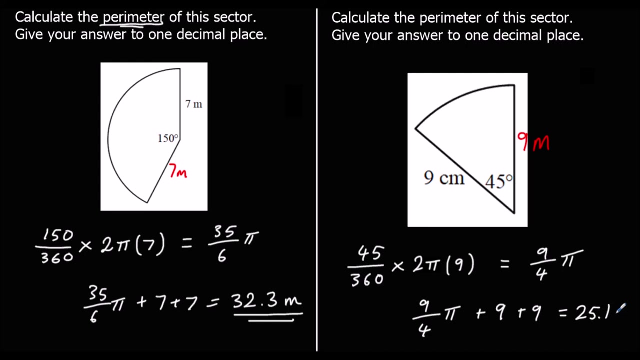 of 2 times pi times 9 is 9 over 4 pi and we're going to get that answer. it's in our calculator and we're going to add on two nines for the perimeter. so the answer plus two nines to 1 decimal place is 25.1 and it's in centimeters: 25.1 centimeters. 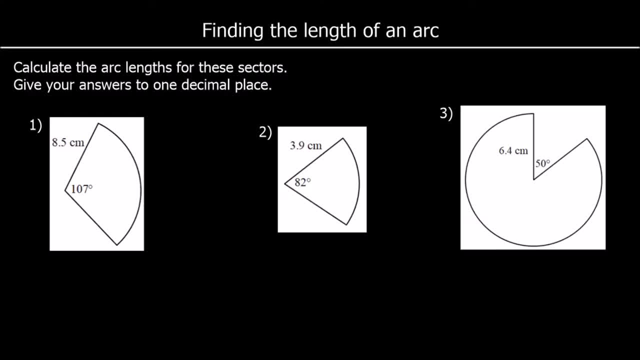 and to finish up, we've got three questions: calculate the arc lengths for each of these vectors. so for the first one, calculating the arc length, let's get rid of the unnecessary��etrains about the ops here. arc length, what fraction of the circle have we got? We've got 107, three-sixtieths of the. 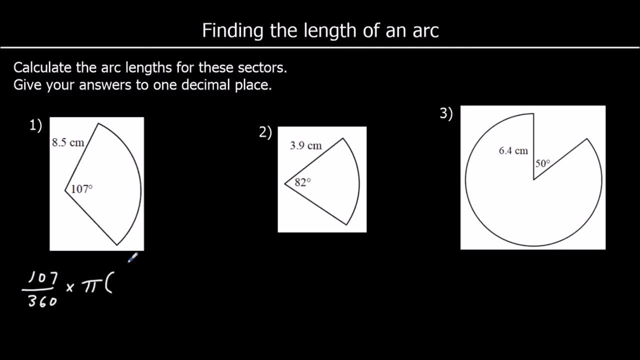 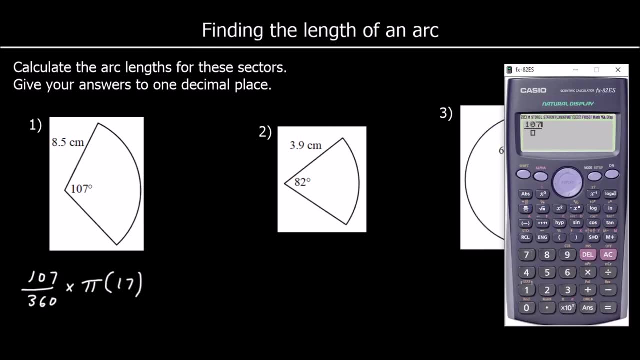 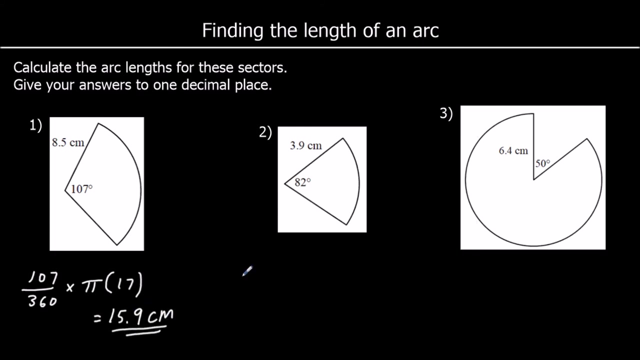 circumference, which is pi times the diameter. two 8.5s are 17.. So we're going to type this into the calculator and give our answer to one decimal place. So 107, three-sixtieths times pi times 17.. So to one decimal place, that's 15.9.. And that is in centimetres For. 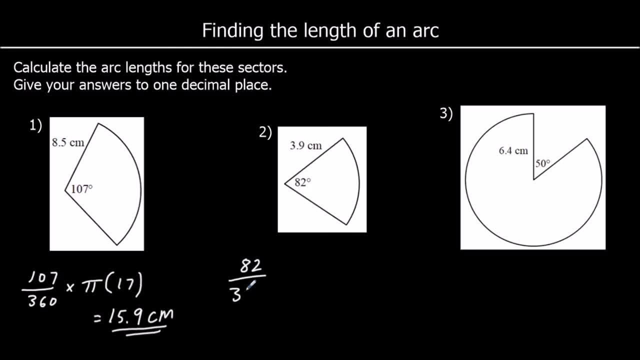 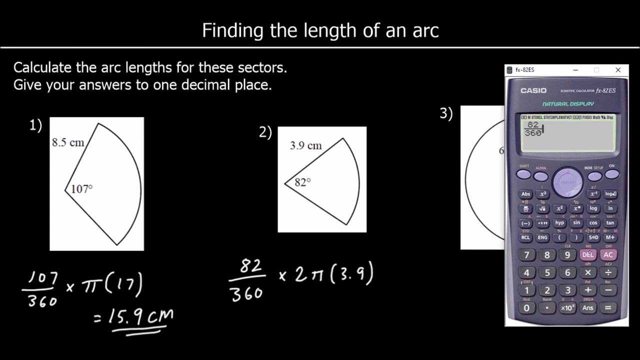 question two: We've got 82 three-sixtieths of the circumference And we use two times pi, times the radius. So this fraction of the circumference again, type it into the calculator And we're going to give our answer to one decimal place.